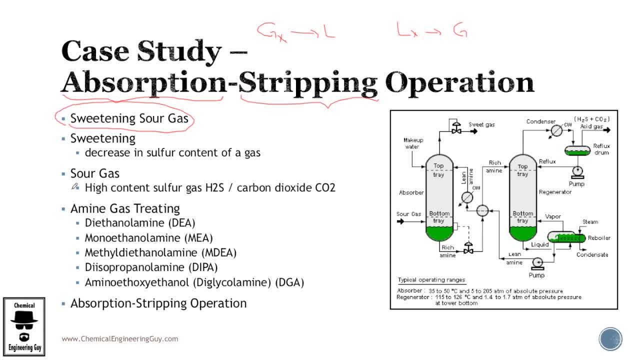 the sweetening of sour gas. Let me explain to you. Sour gas is any high content sulfur gas, typically hydrogen sulfide, and it can also account for the carbon dioxide. They are said to be acid gases because they can form acid in aqueous material, So H2S. 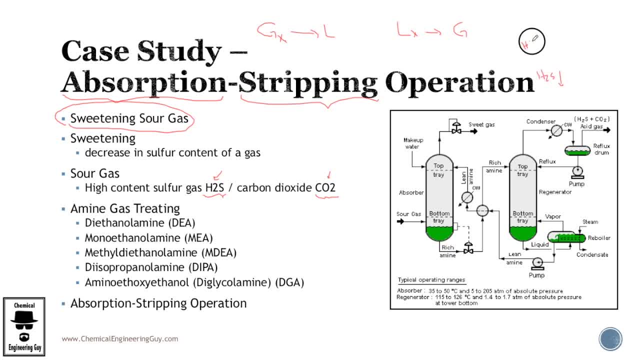 can go in water and act as an acid. The protons will be delivered and CO2 can form carbonic acid, which you know will throw away also protons, which is the acid. So why are we interested in removing this? Because, first things first, this is a high contaminant. 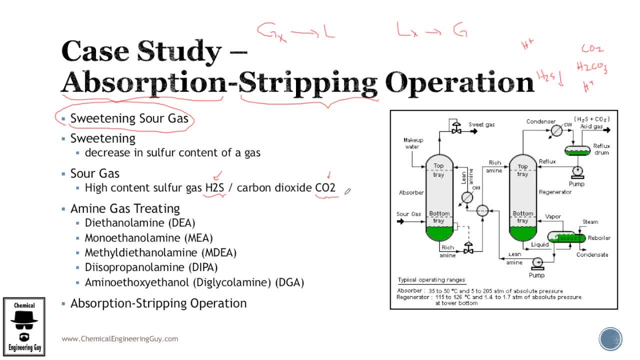 And this is also a high- well, not that high, but also a contaminant. What we want to do is to remove these from our gases. So sour gas can be a hydrocarbon mix, Cxy. You can be talking about natural gas petrol. 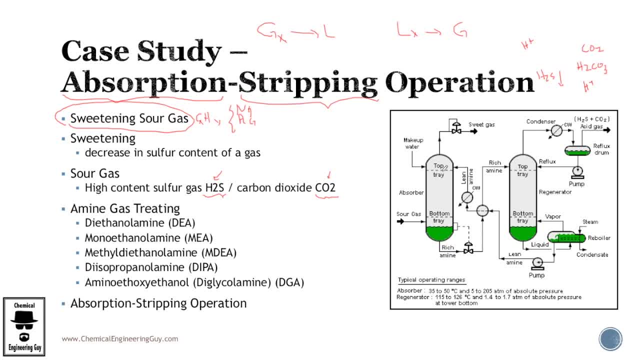 lithium, liquefied gases, whatever type of gas you are interested, not only those, but those are the common ones. you can remove. the sourness, So sweetening as you can imagine, is the decrease in such quantities. What we want to do is to remove this material. This is done via the amine. 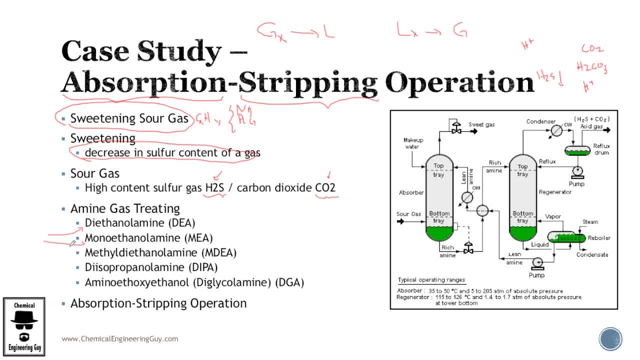 gas sweetening. What happens here is that we add some amine solutions which are going to interact with the acid and they form a complex which is, let's say, removes the hydrogen. so that's the absorption. We've got the liquid, which is the DEA, MEA or so on, and we see these are the two most. 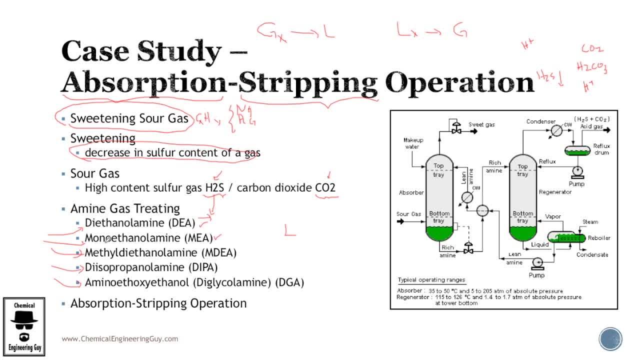 common ones, the ethylamine and monoethanolamine. So what's happening is that there is a gas with X. this is actually reactive amine, because X will react with the liquid, which is the amine to form the LX. So gas is now free to go. this is the chemical. 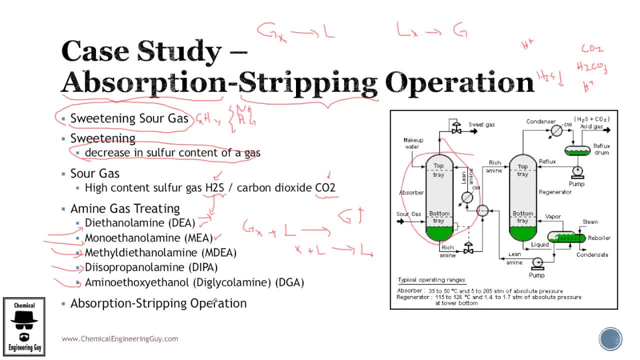 absorption. So this is achieved in the first process. We're going to see this later on, no worries. And the stripping part is, of course, you don't want to throw away this liquid amines, because these are your solvent, those are your raw materials. So what happens? 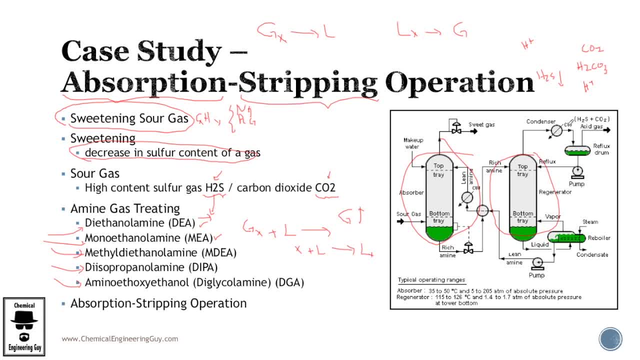 is that you bring them here. you try to condense all the amine possible, which is a lot and some is not, as well as the acid gases such as hydrogen sulfide and CO2.. So these are non-condensable material. the liquid goes back, the low-acid amine reacts with the high-acid amines and 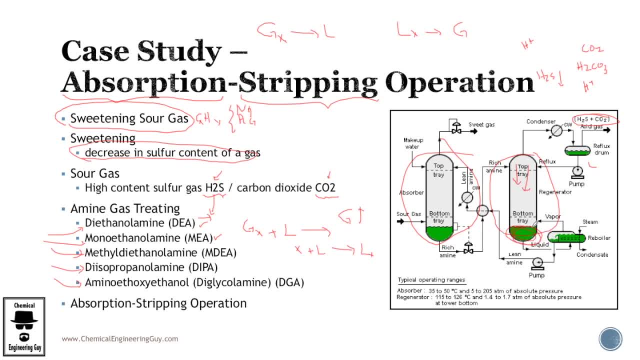 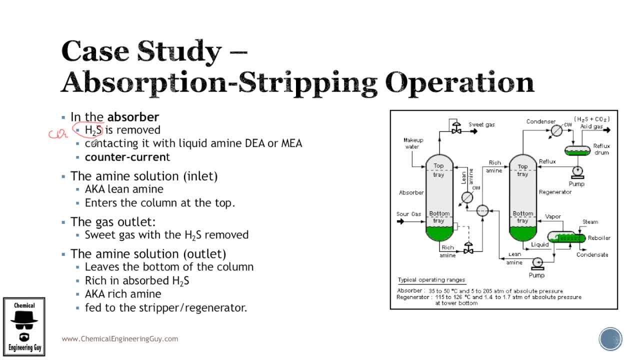 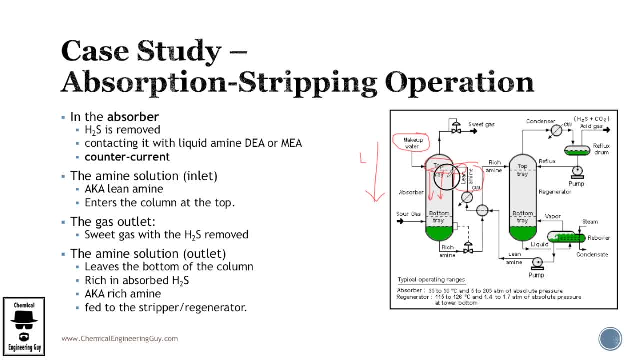 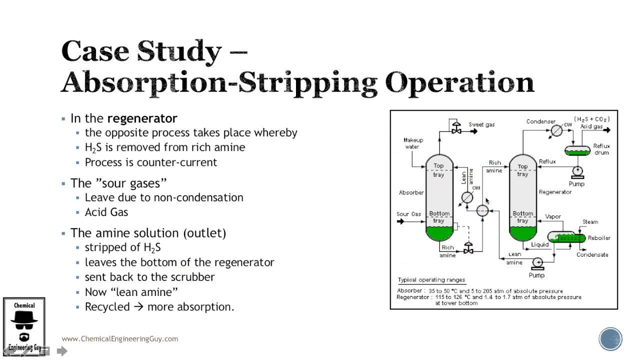 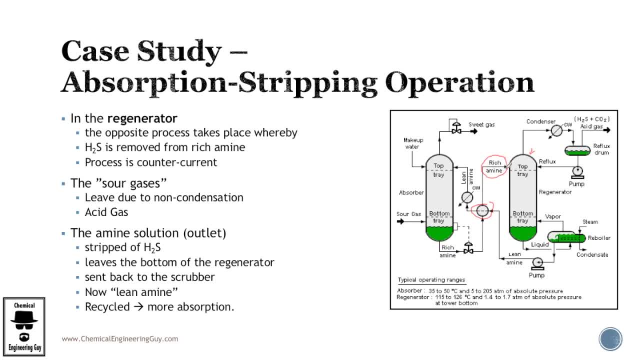